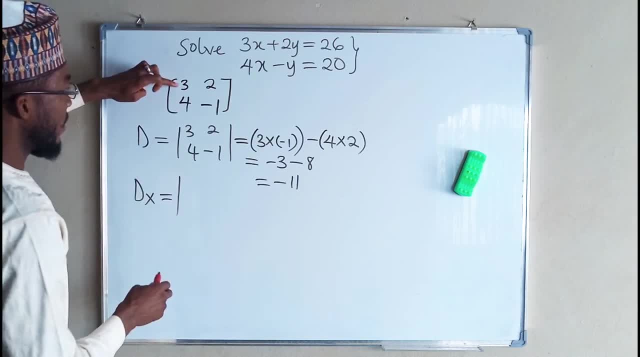 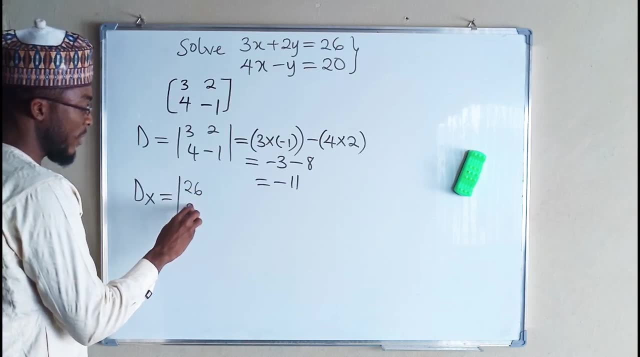 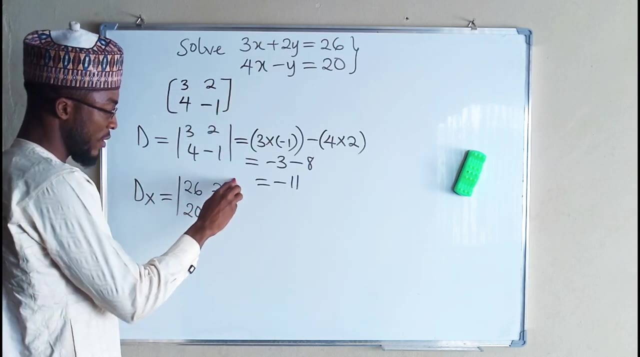 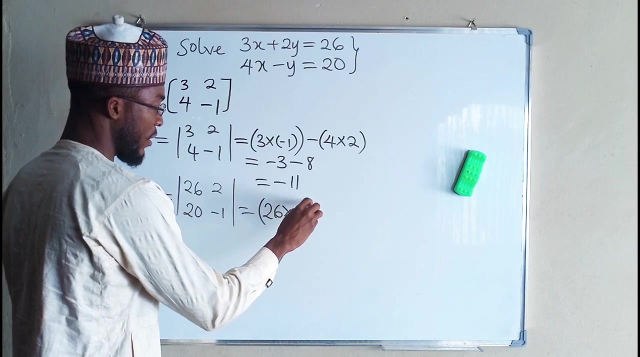 The determinant with respect to x. you need to replace the coefficient of x with the constant times. The constant times are 26 and 20.. And the coefficient of y remains constant, And this will give us 26 multiplied by negative, 1 minus 20 times 2.. 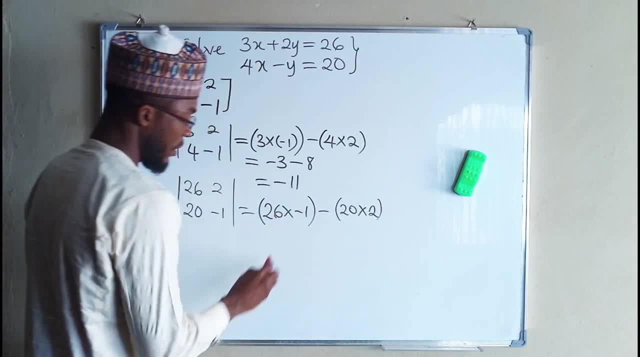 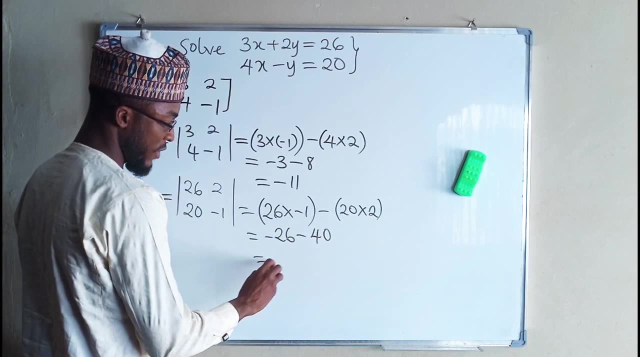 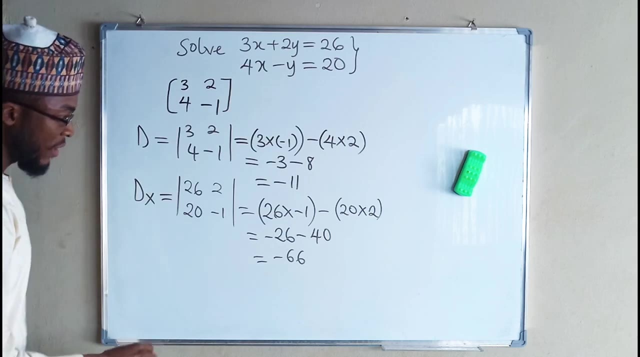 This is negative 26 minus 40. And this will give us negative 66.. This is the determinant with respect to x. You need to find the determinant with respect to y, And this is: You keep the coefficient of x constant 3 and 4.. 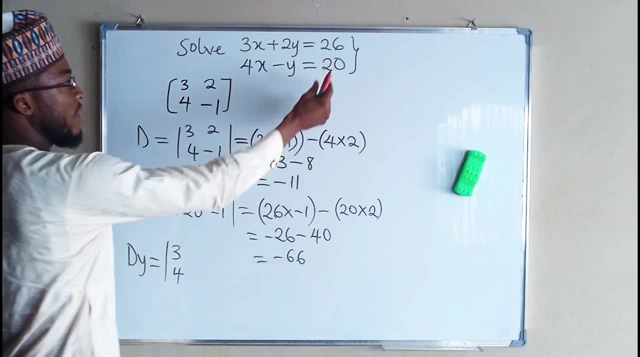 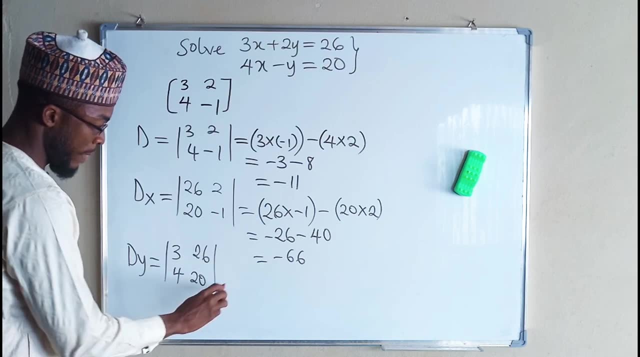 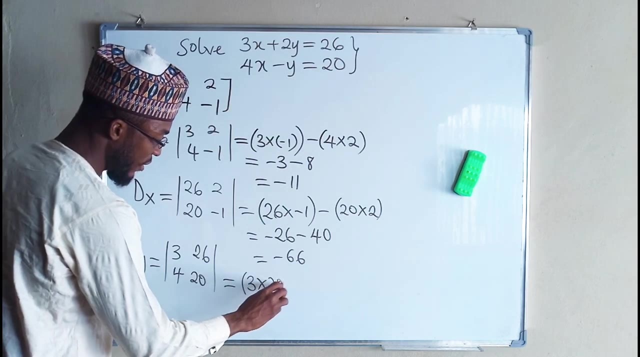 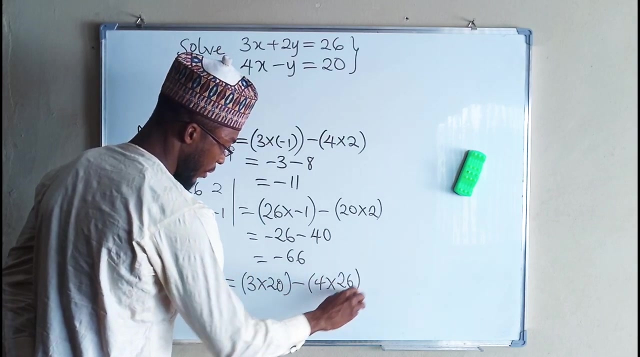 Then, instead of the coefficient of y, you replace them with the constant times 26 and 20.. And this will give us 3 times this Times 20.. Minus 4 times 26. And this is equal This time. this will give us 60.. 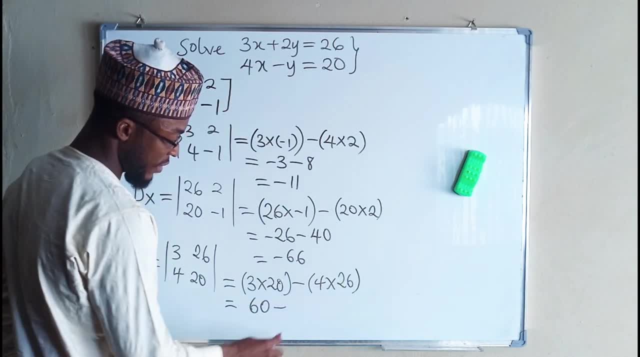 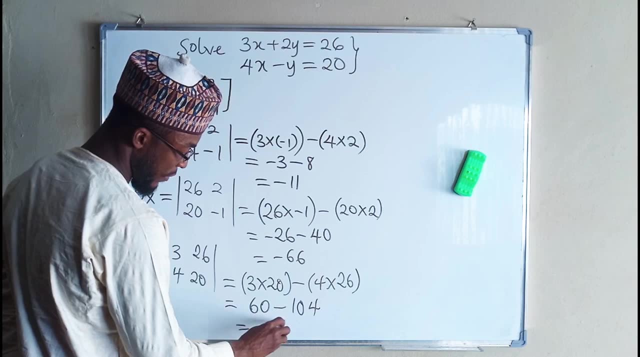 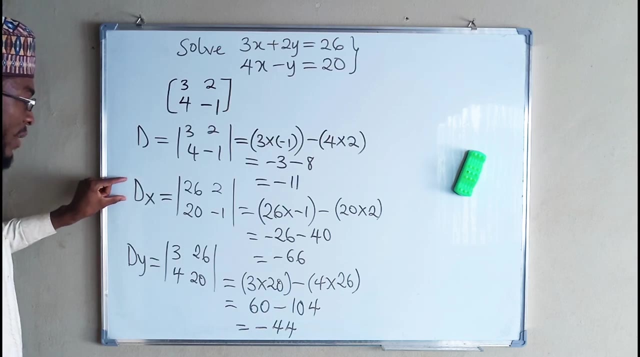 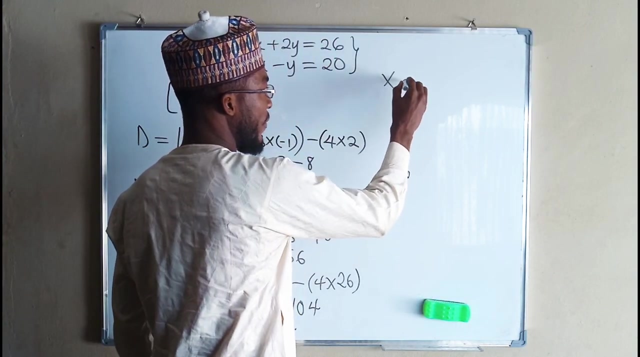 Minus 4 times 26 is 104. And this will give us negative 44.. So we have found the determinant with respect to x and the determinant with respect to y. So the value of x, The value of x, is equal to dx divided by d. 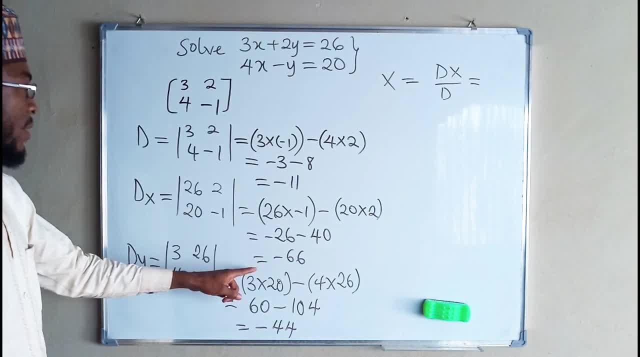 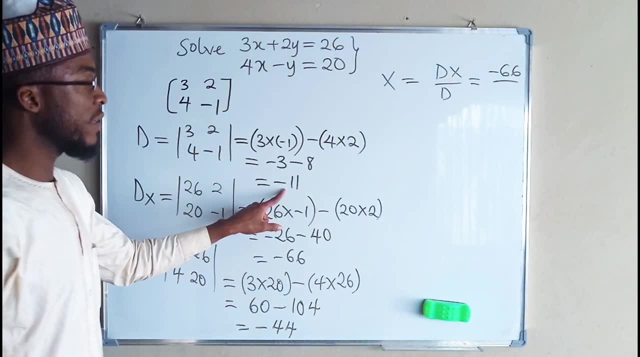 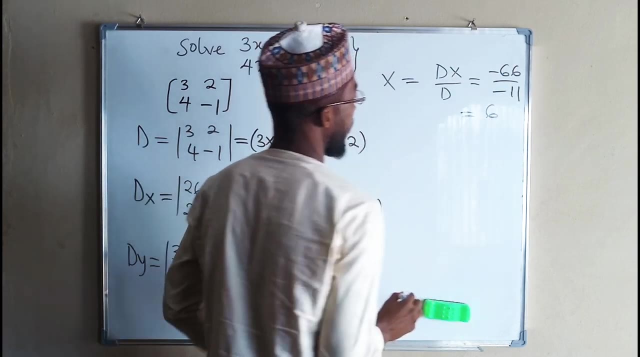 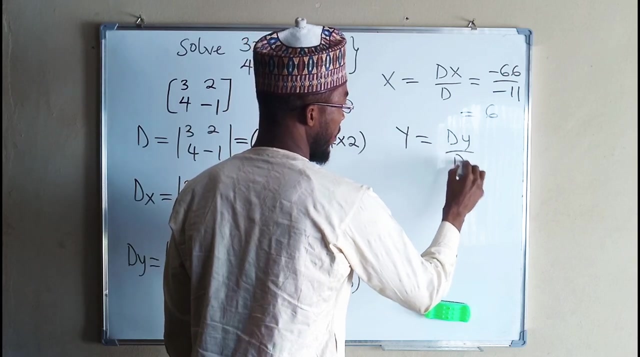 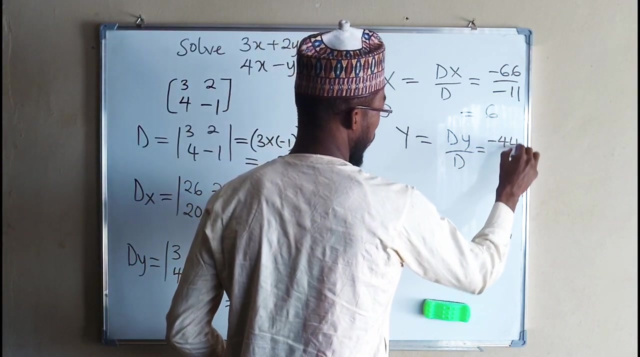 And our dx here is negative 66.. Negative 66 divided by d And d is negative 11.. Negative 11. And this is equal to 6.. To find y you need to divide dy over d, And dy is negative 44..